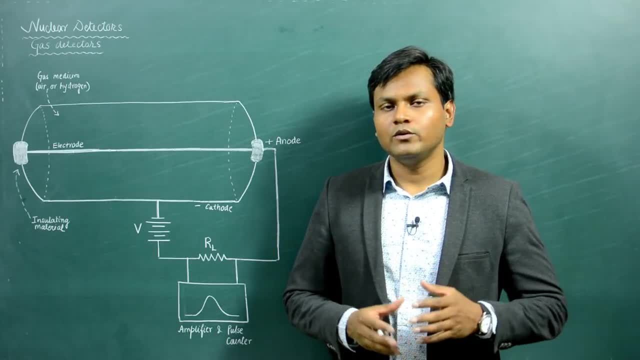 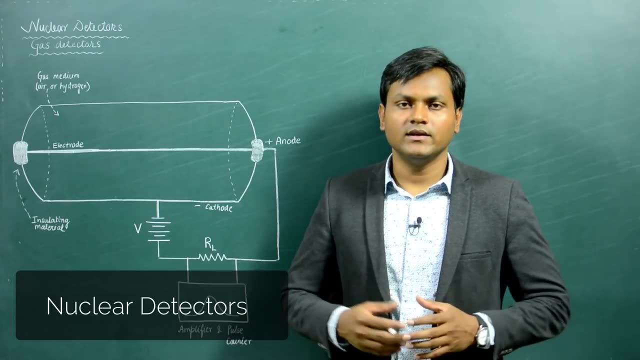 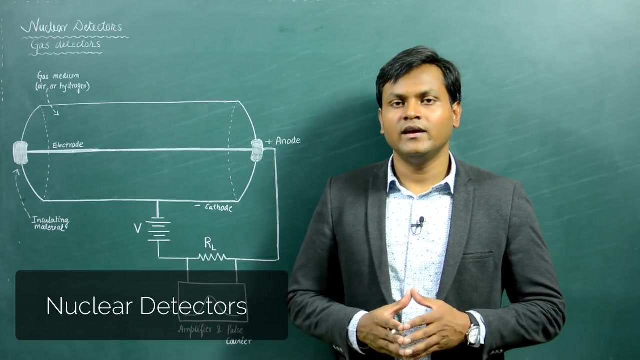 Hi, welcome back to my video once again. So in this video I want to talk about nuclear detectors. So nuclear detectors are special kinds of instruments that can detect nuclear particles like alpha particle, beta particle, gamma radiation, etc, etc, and can also determine their energy momentum direction etc. So out of the many different kinds of nuclear detectors there is a 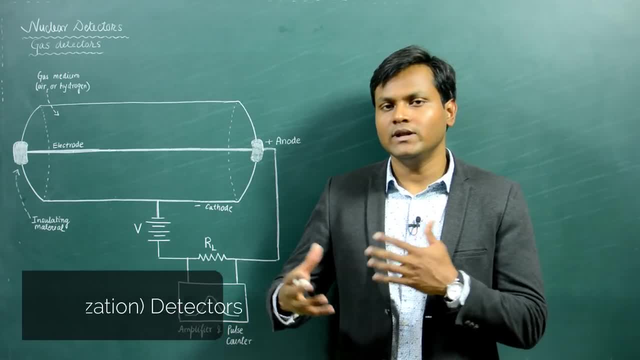 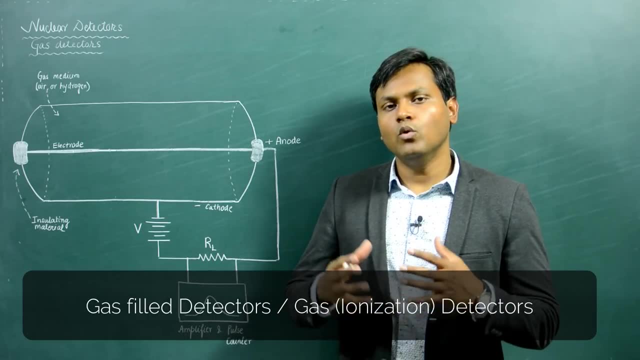 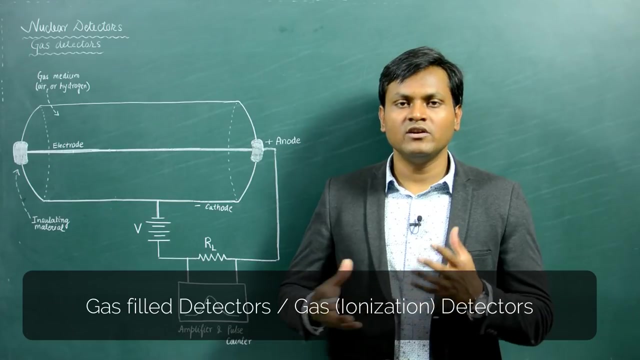 class of nuclear detectors known as gas-filled nuclear detectors or gas chambers, and in this video I want to discuss the general principle and working mechanism of these kind of gas-filled nuclear detectors. So by the end of the video you'll understand not only the general principle, 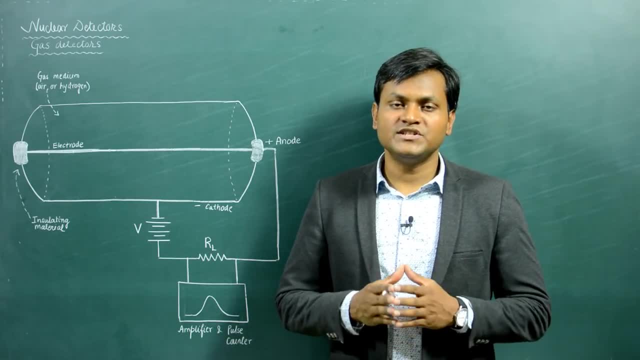 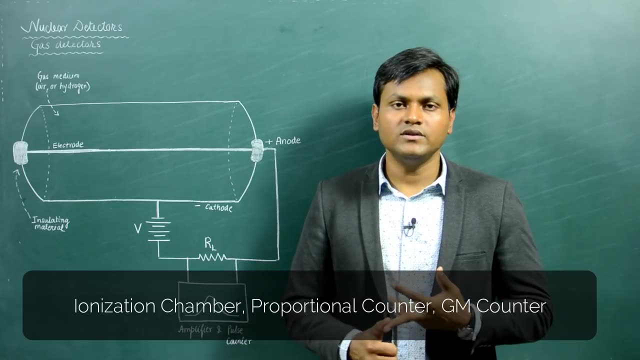 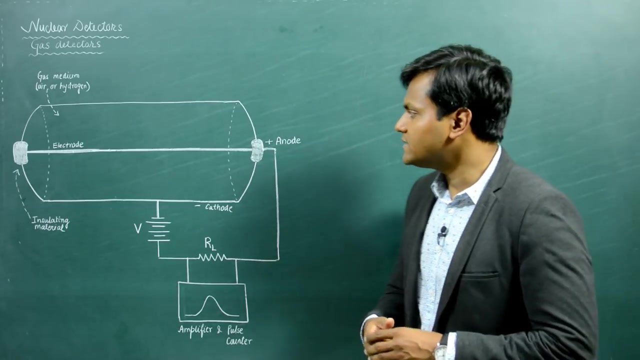 with which these detectors work. but you should also be able to distinguish between different kinds of gas-filled nuclear detectors, like ionization chambers, proportional counters, gigamiller counters and so on and so forth. So let's begin. So here we have a general construction of those kind of nuclear detectors. 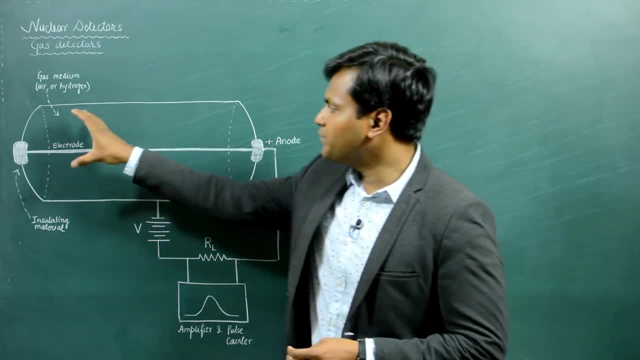 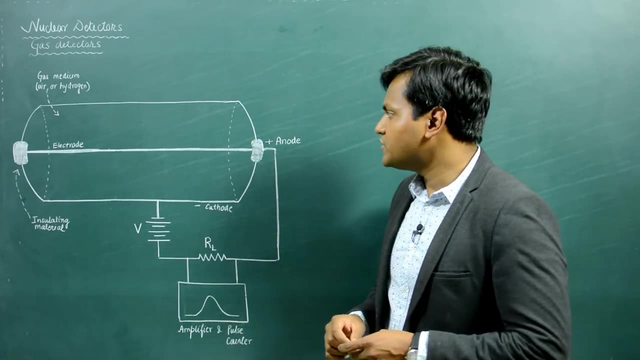 So here you basically have a metallic cylinder which is hollow from the inside and it is filled with some kind of a gaseous medium like hydrogen air at one atmospheric pressure, And along the center of the cylinder you have a metallic electrode which is passing through it. Now 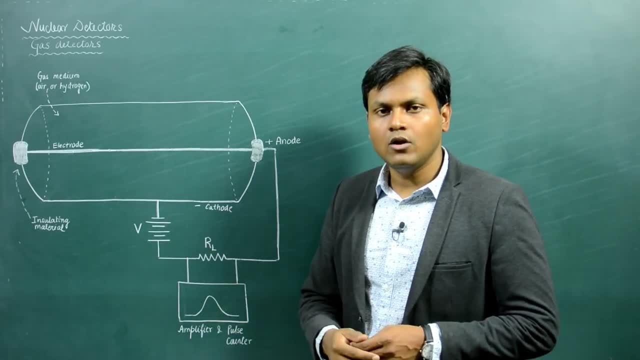 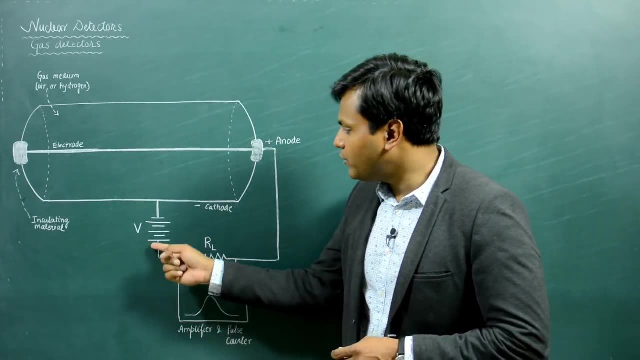 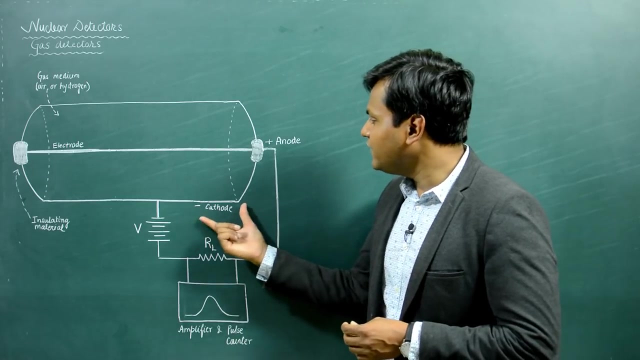 this cylindrical surface is connected to some negative terminal of a voltage supply and the metallic electrode passing through the center is connected to a load resistance which is again connected to the positive terminal of the same power supply. Now, to prevent this positive metallic electrode from touching the negative, 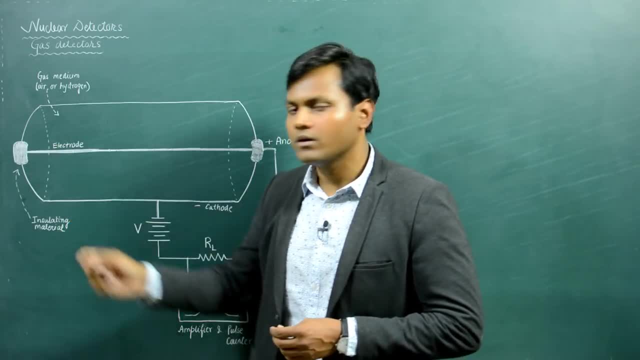 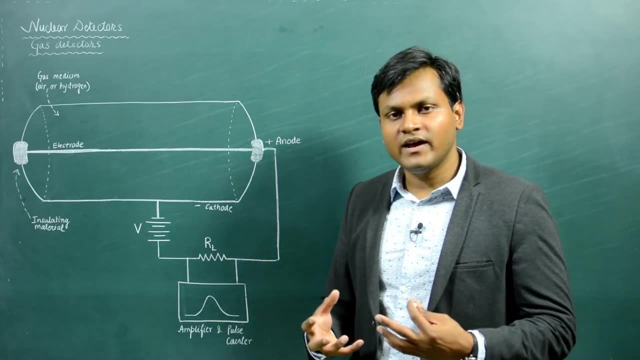 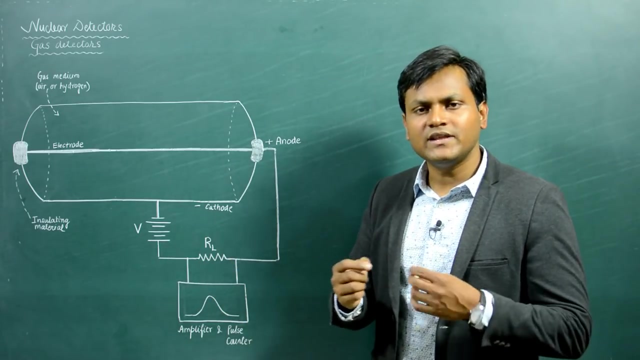 metallic surface, there is some kind of an insulating material. Now, across the load resistor, you have some sort of electronics which is connected to it, like some kind of an amplifier or a pulse counter that can basically detect the potential drop that is happening across RL and measure the amount of current which is passing through RL. So what is the? 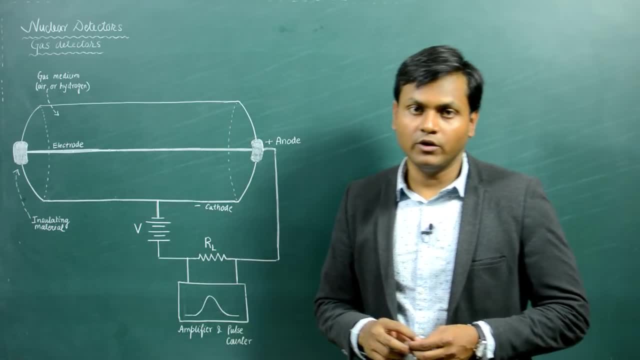 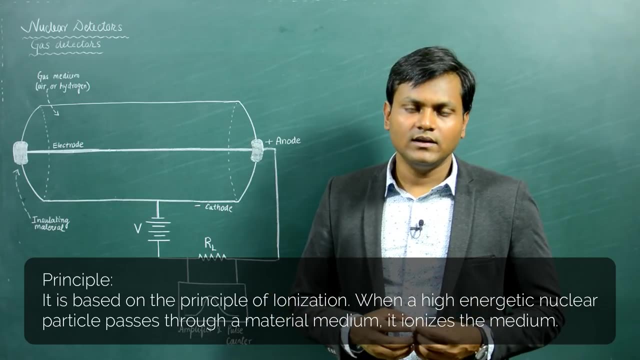 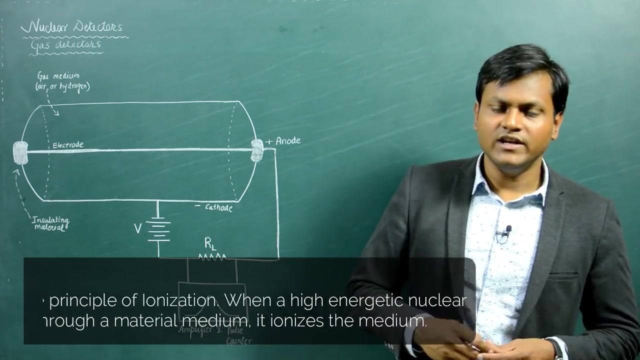 principle on which this kind of a nuclear detector is based upon. It is based upon the principle of ionization. So when a high energetic nuclear particle passes through some kind of a material medium, it basically ionizes the material medium. Now, what is ionization? It is quite simple So. 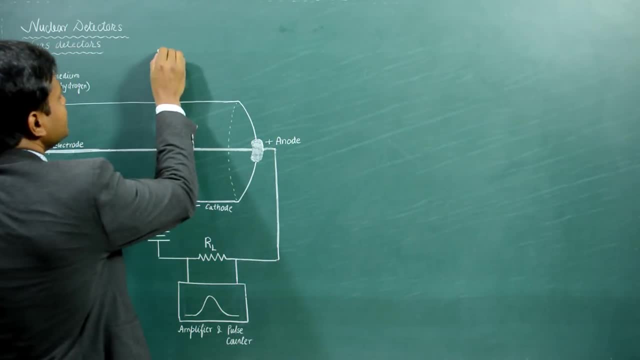 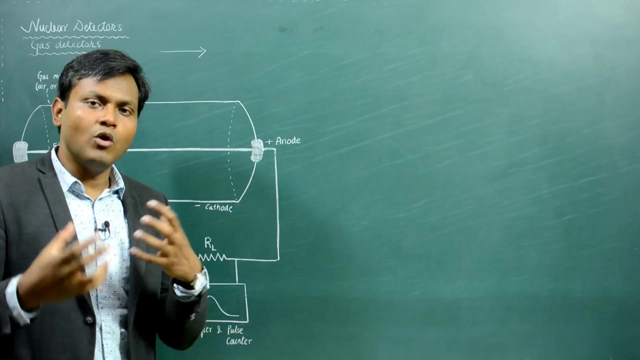 let's take the example of, let's suppose, an alpha particle which is passing through some kind of a material medium. Now, alpha particle is quite energetic and it collides with the molecules and of that material medium and with every single collision it basically transfers some of its. 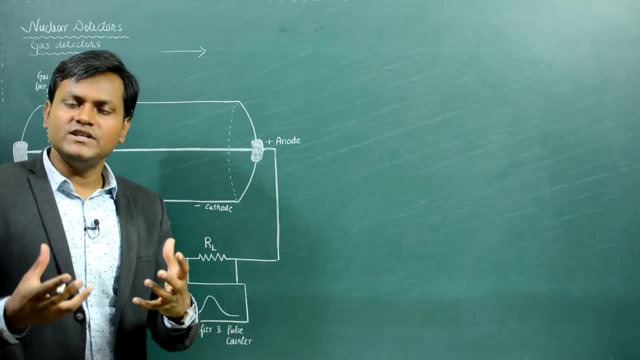 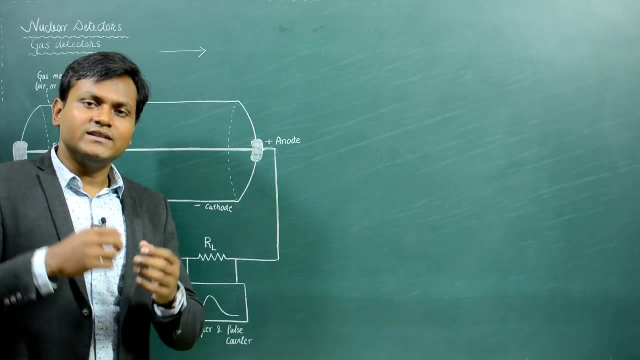 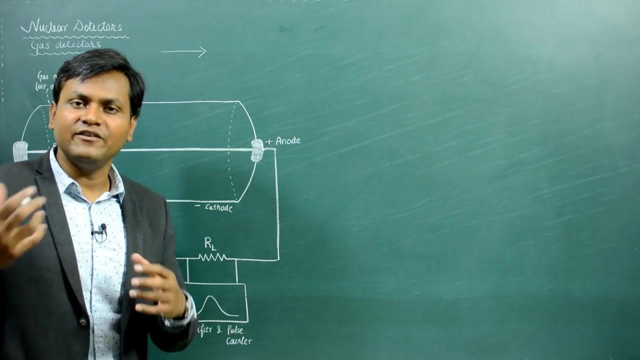 energy to the molecules of the material medium, and this energy is basically absorbed by the electrons in the outermost shells of these atoms and molecules. and if the energy is sufficient enough, the electrons will absorb that energy and become free from the atoms and molecules, thus creating a positive ion and a free electron. Now, this kind of collision happens many, many number. 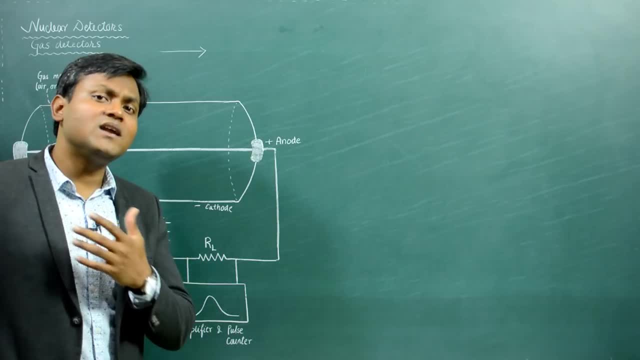 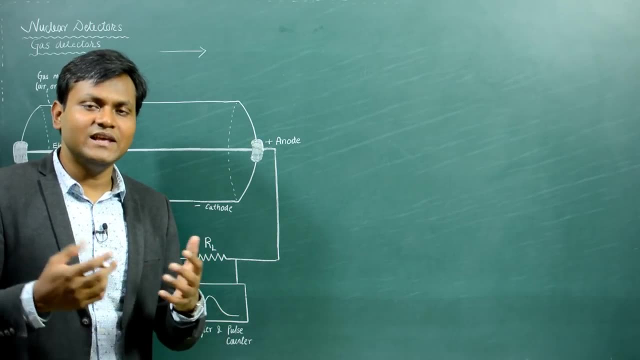 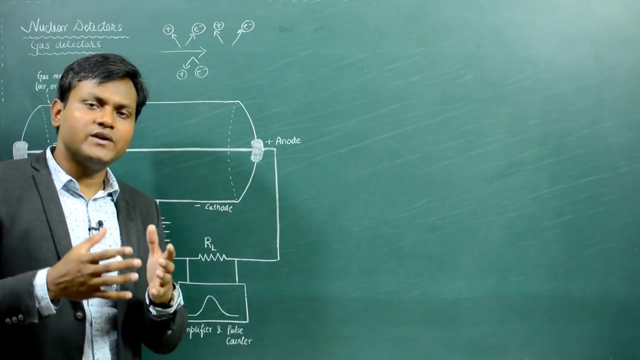 of times so along the trajectory of an alpha particle or other high energetic beta particle or gamma radiation. due to many number of collisions, large number of pairs of positive ions and free electrons are created. So when a nuclear particle enters a material medium, it basically leads to the creation of pairs of ions and free electrons. The greater the energy of the 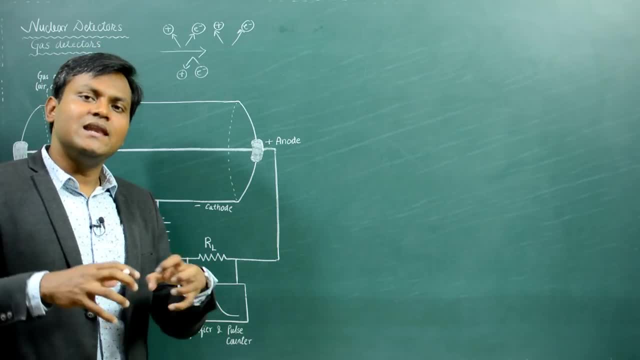 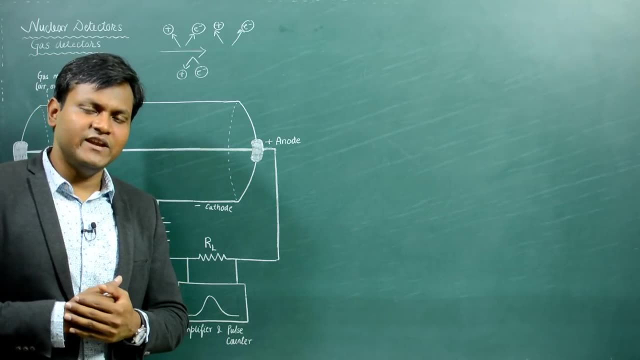 nuclear particle, the larger is going to be the ionization and larger is going to be the number of positive ions and free electrons which are created. Now, what is the difference between a nuclear particle and a free electron? What happens when these positive ions and free electrons are created in the first place? They 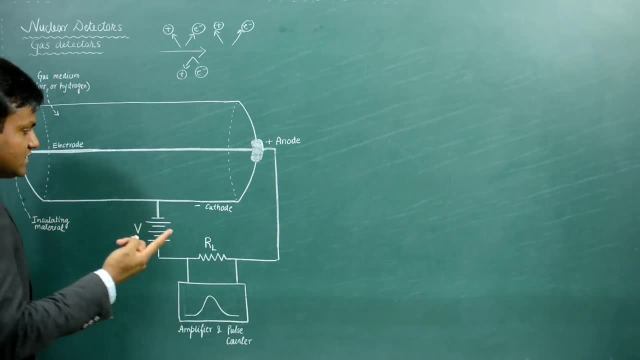 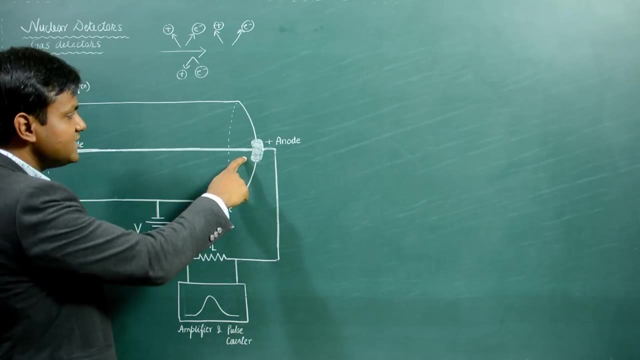 are subjected to an external electric field. So, as you can see here, the metallic surface is connected to the negative terminal of the battery, while the metallic electrode passing through the center is connected to the positive terminal. So basically, you will end up getting an electric field along. 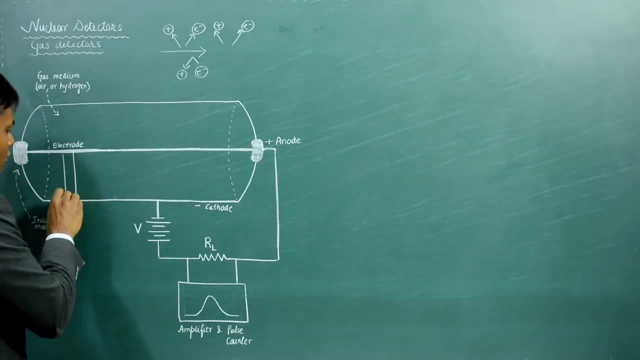 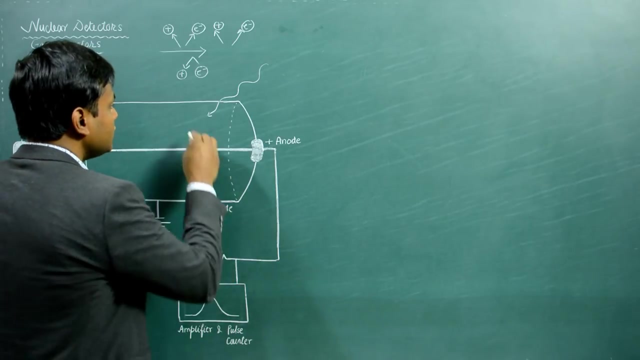 this particular direction. So you will get an electric field which is directed from the metallic electrode towards the metallic surface. So every time some kind of an external nuclear radiation enters this material medium and leads to the creation of positive ions and free electrons, then these charged particles are. 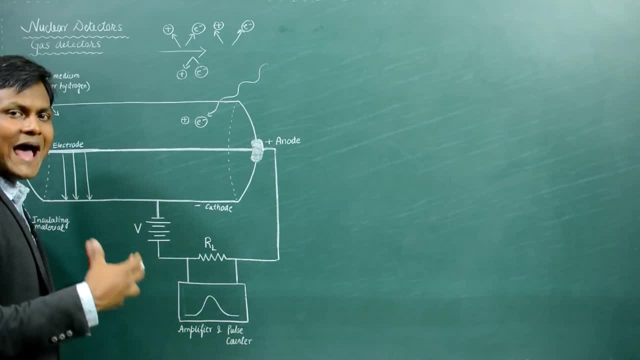 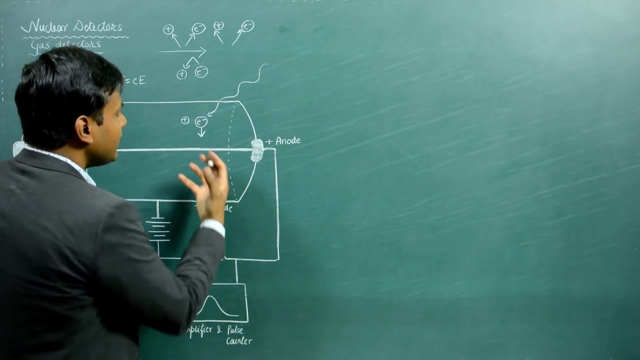 now subjected to this electric field. So what happens is that this electron will now experience an electric field towards the metallic electrode and it experience a force where the force is basically given by the electric charge multiplied by the electric field, and then then it will accelerate towards the electrode, while the positive charge will be accelerated. 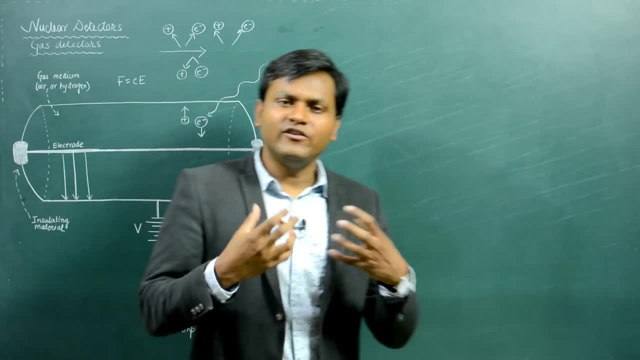 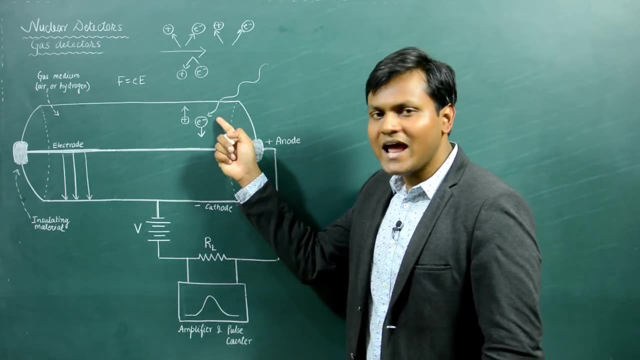 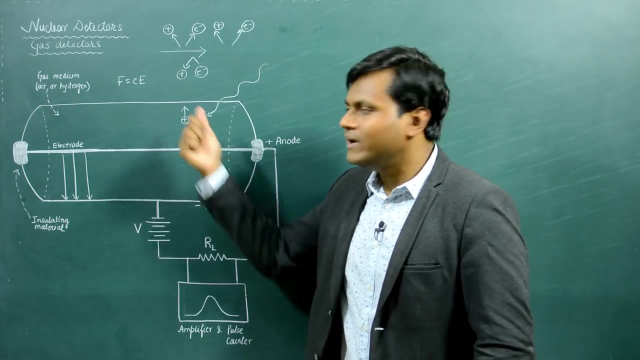 towards the metallic surface. so all the ions and free electrons which are created during the primary ionization process when an external nuclear radiation interacts with the material medium. so these primary ions will be attracted towards opposite polarities of the metallic electrode and the metallic surface. so after some time, all of these free ions which were created. 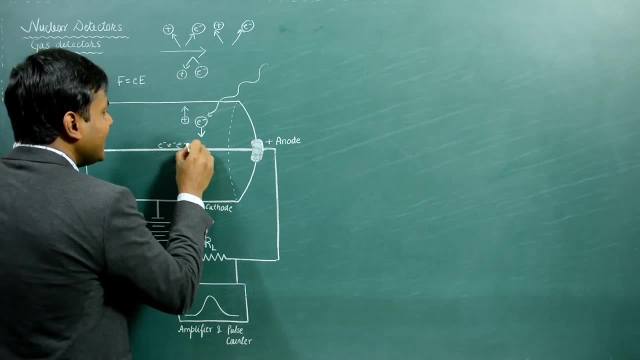 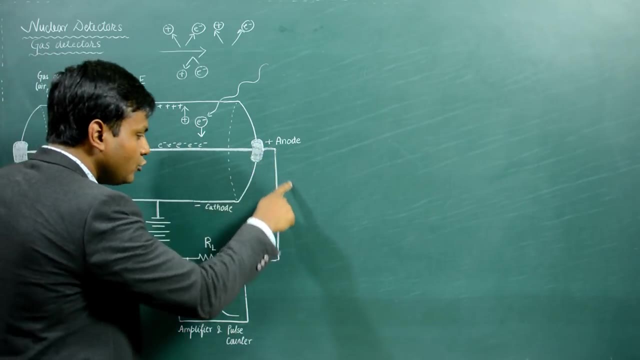 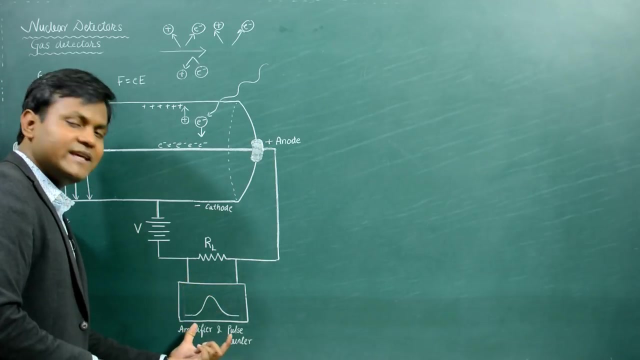 will get accumulated along the metallic electrode as well as the metallic surface, and all these electrons which get accumulated on the metallic electrode travel through the circuit and they basically lead to a potential drop across rl. and this potential drop across rl is detected by the electronics as proof of the existence of an external nuclear particle. so the electrons 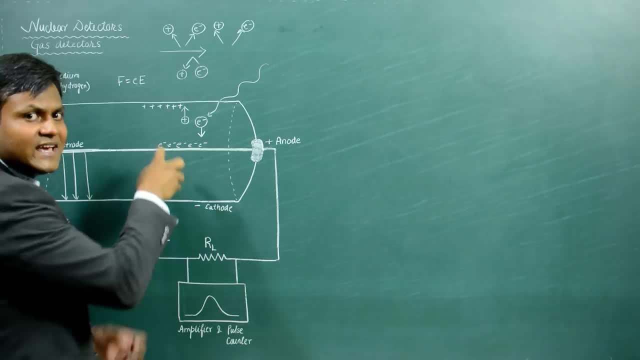 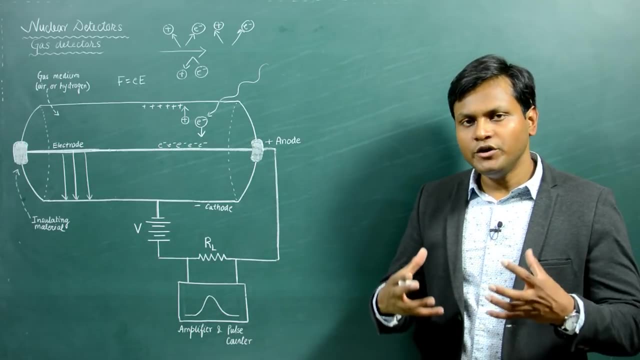 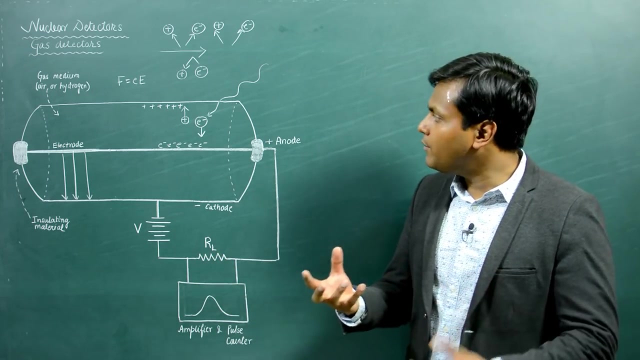 complete the circuit and then get absorbed by the positive ions, which become neutral again, thus bringing the entire configuration back to the original configuration, back to its original state. now it is important to note that the size of the current pulse which is detected across this load resistance is dependent upon the energy of the 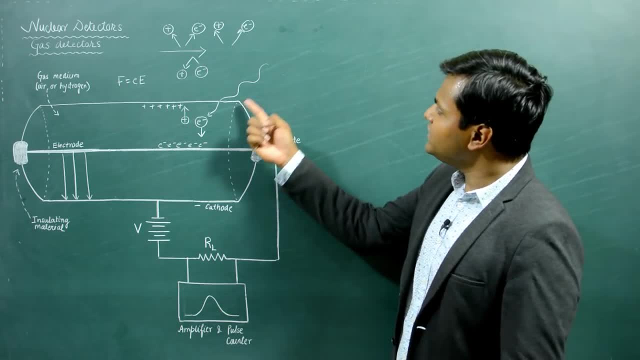 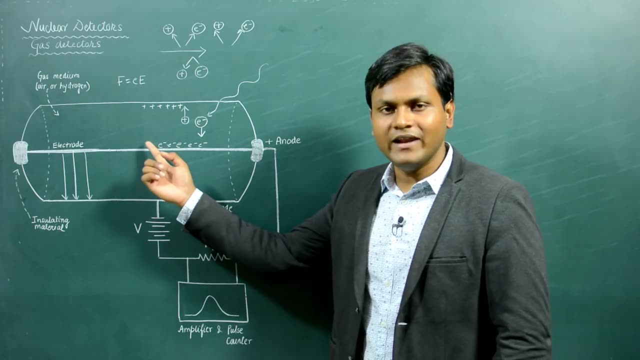 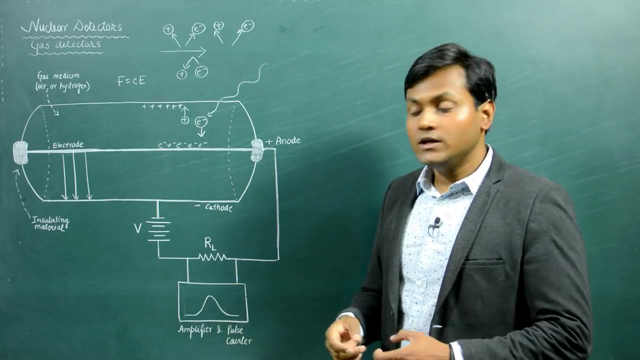 incident radiation. why? because if the energy of the incident radiation is very high, then that would lead to a huge amount of ionization, which will create a large number of electrons and free ions, which will end up creating a greater amount of current, does leading to a bigger current signal. 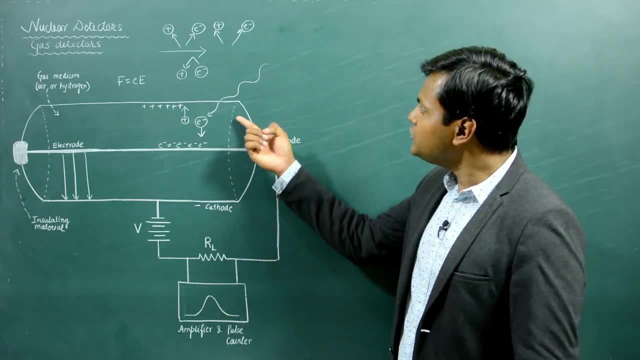 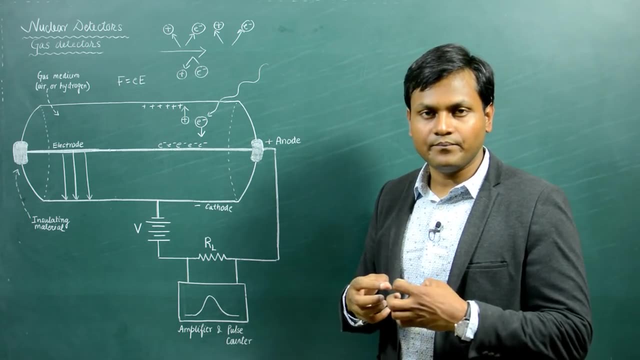 so a bigger rider current pulse will automatically mean that the energy of the incident radiation is greater, and the smaller current pulse will mean that the energy of the incident radiation is lesser. Now there is another variable which is involved here: the voltage of the battery. What happens to this particular process? 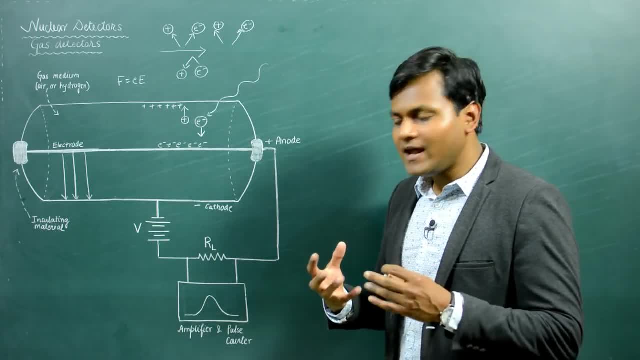 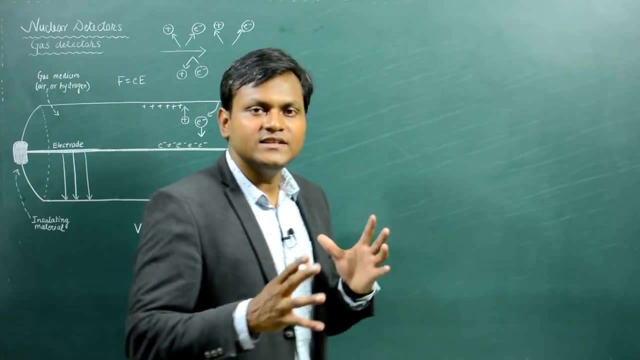 when we change the voltage of this particular battery. So to understand how the size of the current pulse changes with respect to the voltage of the battery, as well as the energy of the incident radiation, let's look at this particular graph here So to understand how the size of the 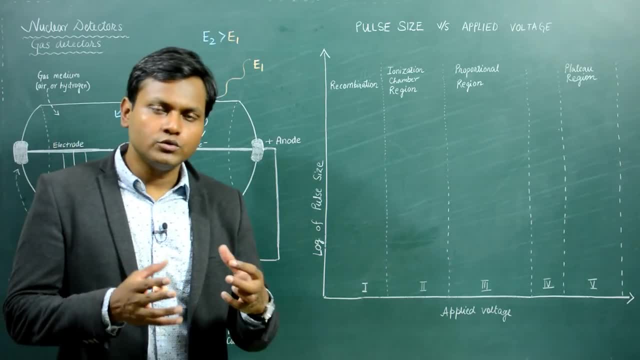 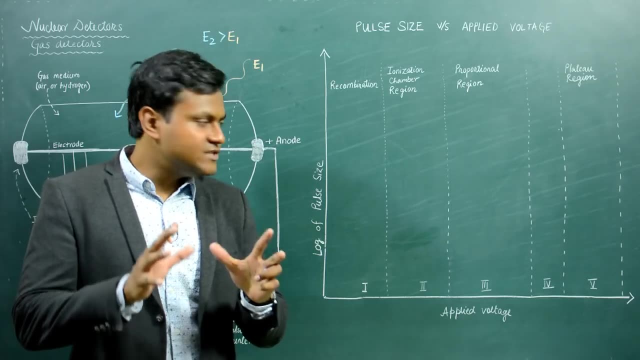 current pulse changes with the applied voltage, and also to distinguish between different kinds of nuclear detectors like ionization chambers, proportional counters and gigameter counters. let's look at this graph here, All right. so in the x-axis you have the applied voltage of the 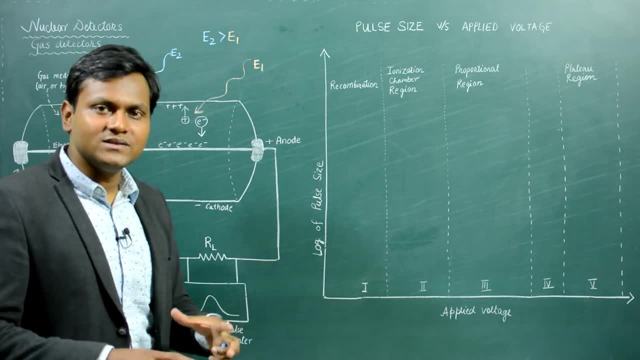 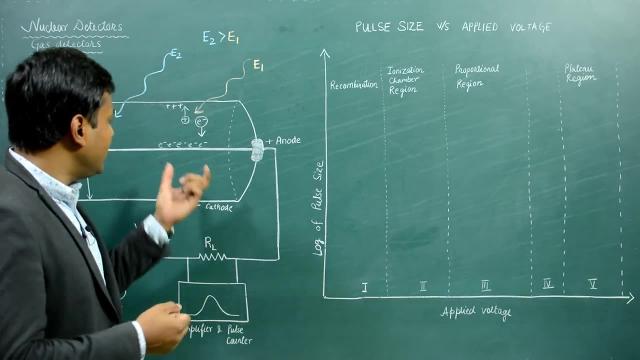 battery and in the y-axis you have the log of the pulse size. Now, when the voltage is very, very less, in that case the electric field will be very, very low and the voltage will be very, very low and the electric field will be very, very low and the electrons and the ions produced by ionization will not experience huge amount of. 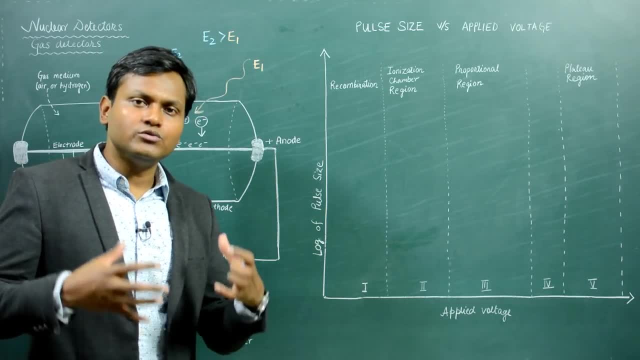 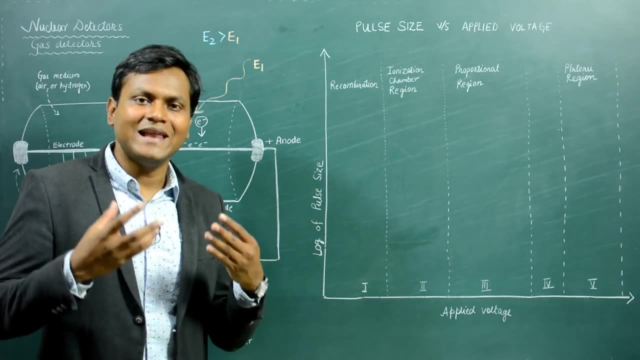 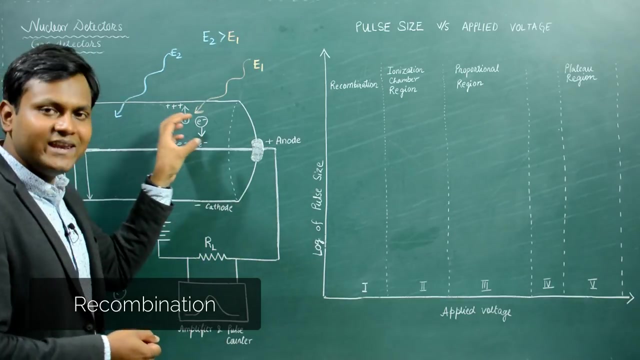 acceleration. Therefore, what is going to happen is that, due to thermal motion, these electrons and the positive ions will come back together and recombine to form neutral atoms. This process is known as recombination. So recombination is a process in which the ions created by the 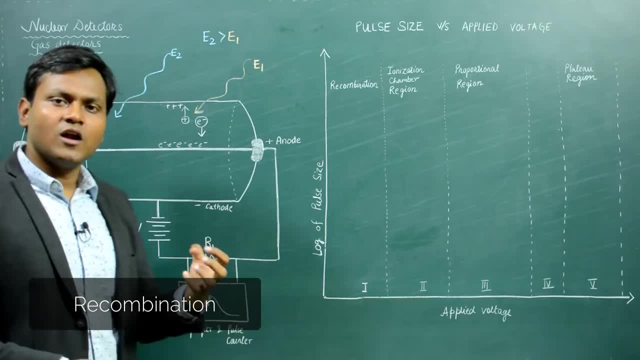 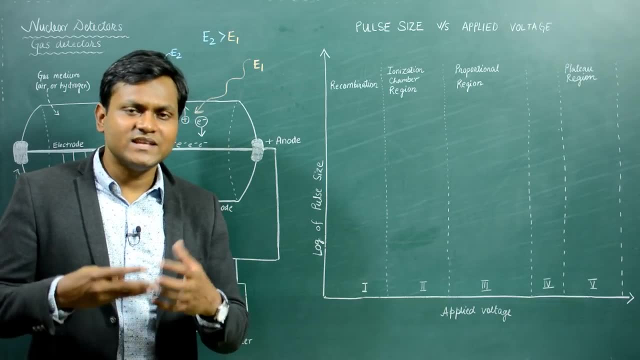 ionization, due to some external nuclear particle, due to thermal motion, come back together and recombine to form neutral atoms. So once they become neutral atoms they are useless and they do not contribute towards the current in the load resistance at all. So when voltage is very less, 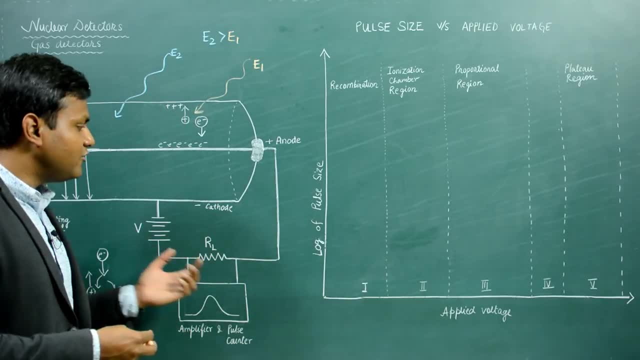 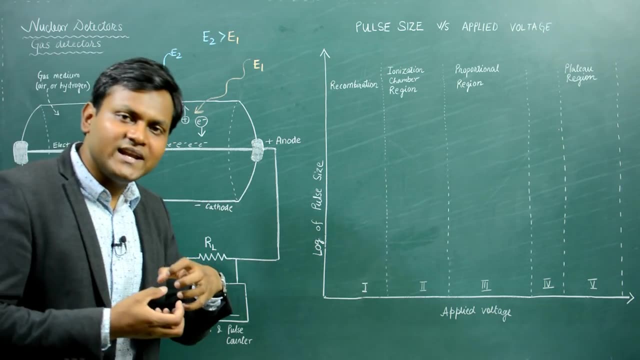 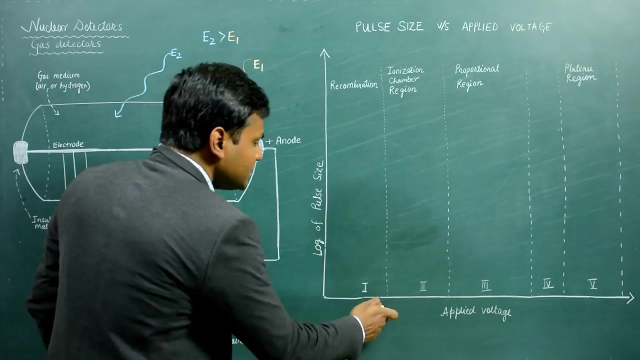 recombination is quite dominant. but when voltage of the battery is increased, then recombination becomes less and less, because the moment electrons and ions are formed they start getting accelerated towards opposite terminals of the detector. So what happens is that when you have increase in voltage the current pulse also increases. So when the voltage is very less, then the recombination 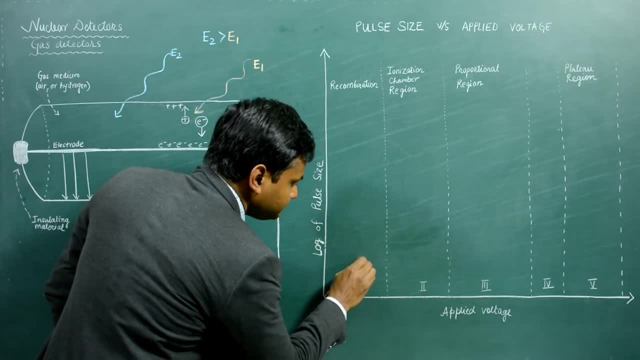 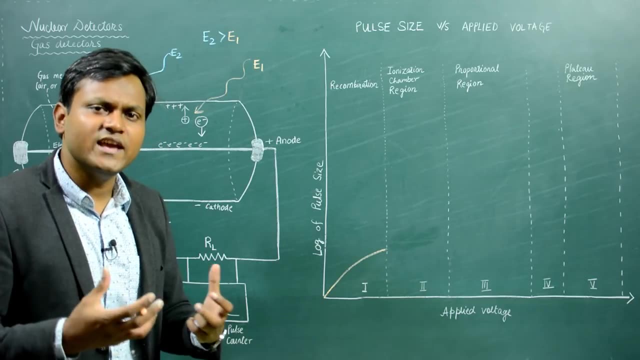 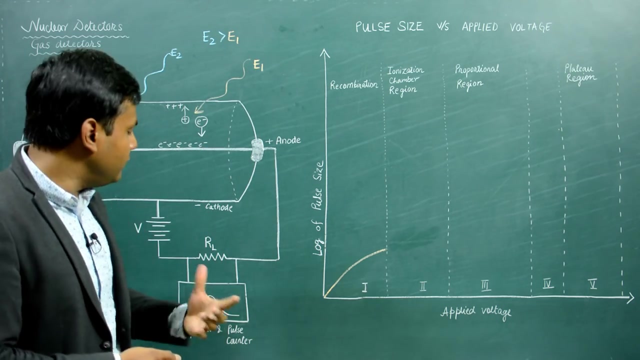 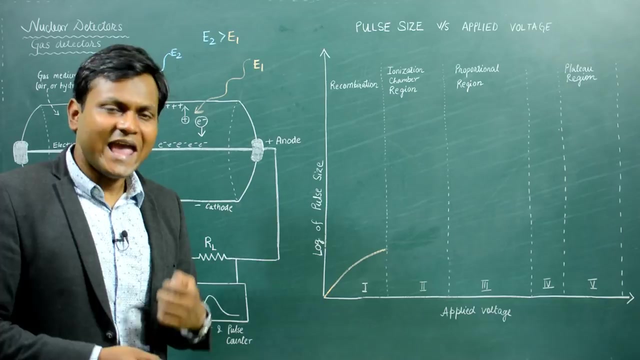 also increases along with it. So this dotted line basically represents that particular voltage in which recombination becomes almost near about negligible and all the electrons and ions created during primary ionization basically end up contributing towards the current pulse. So this is the maximum current pulse possible due to primary ionization and further increase in voltage. 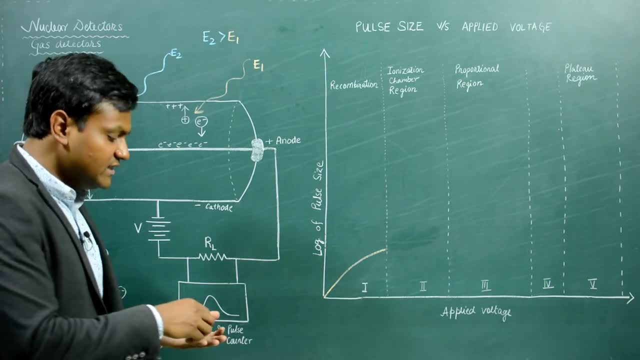 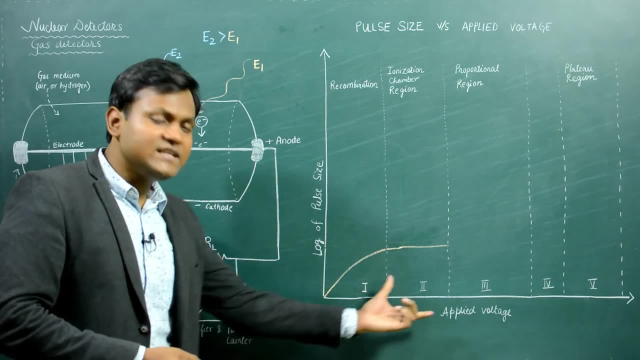 will not contribute towards the increase in the voltage. So this is the maximum current pulse of the current signal. So the first region is distinguished by the presence of recombination, and increasing the voltage decreases recombination and we end up getting the maximum current size possible. 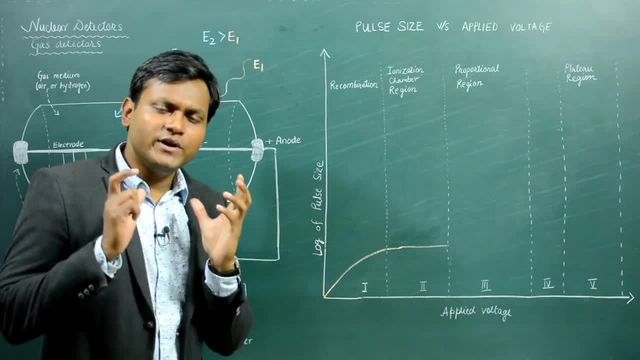 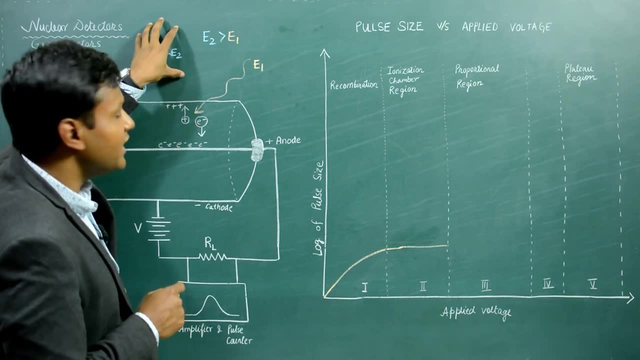 for a particular energy of the nuclear radiation. Now I also want to distinguish between two situations: One situation where nuclear radiation has an energy of E1 and second situation where the nuclear radiation has energy of E2.. Let's suppose E2 is greater than E1.. Now what is going to happen? 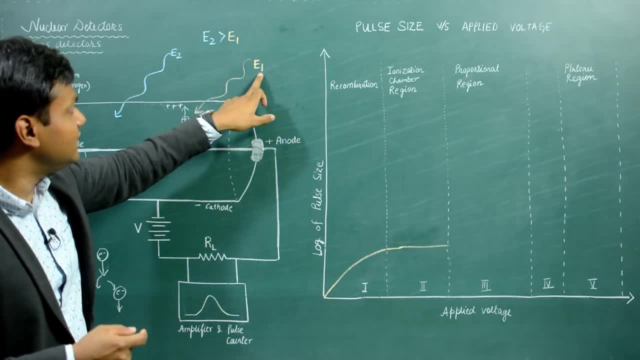 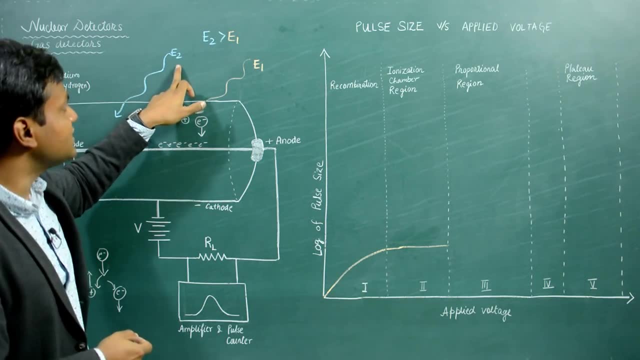 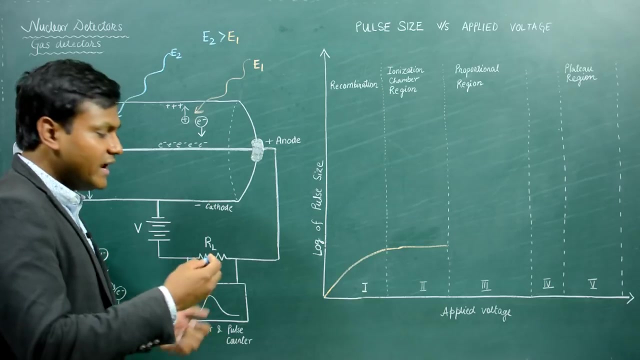 for the case of particle. In this case the ionization will be greater, So the number of ions created will be larger in the case of E2 as compared to E1. So you will see the same sort of behavior for the second particle. However, the current pulse will be greater for the second particle with increase in voltage. 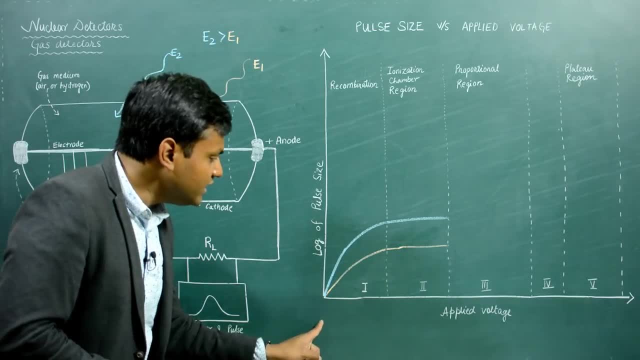 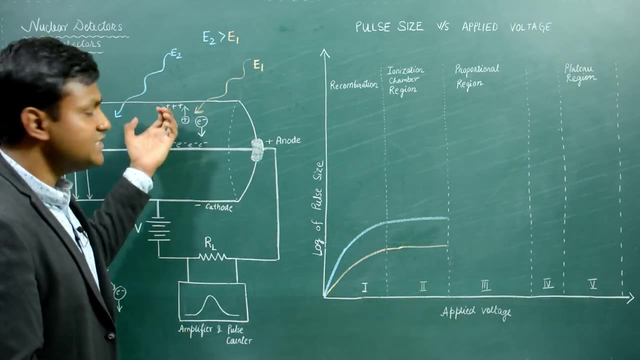 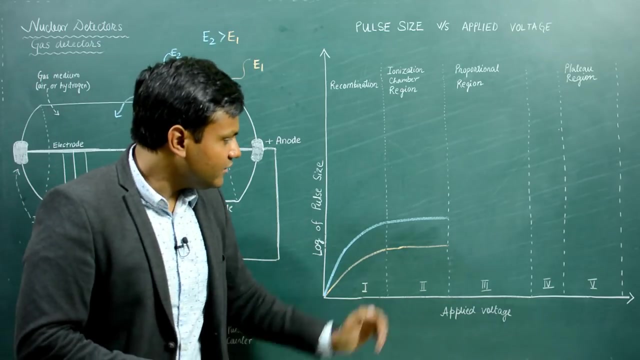 So, as you can see here, in region number one, with increase in voltage recombination decreases and we end up reaching the maximum possible current pulse for the primary ionization, the primary ionization's cost. however, for greater energy of the incident particle, the current pulse will be greater. in the second region, as you can see here, recombination is near about zero and the 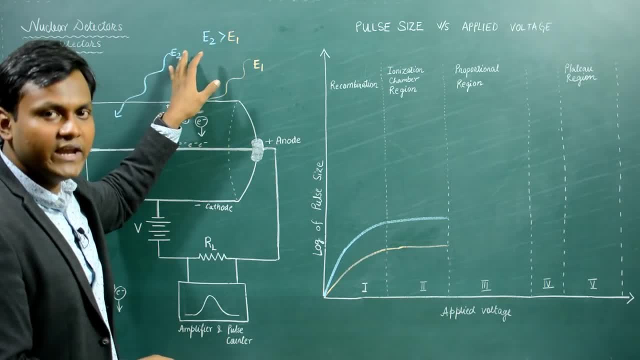 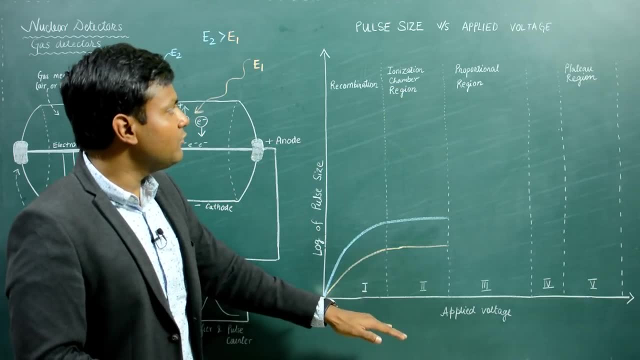 current pulse is purely dependent upon the energy of the incident radiation and it is not dependent upon any further variation in the voltage of the battery itself. so this region is distinguished by ionization chambers. so ionization chambers works in region number two, where recombination is near. 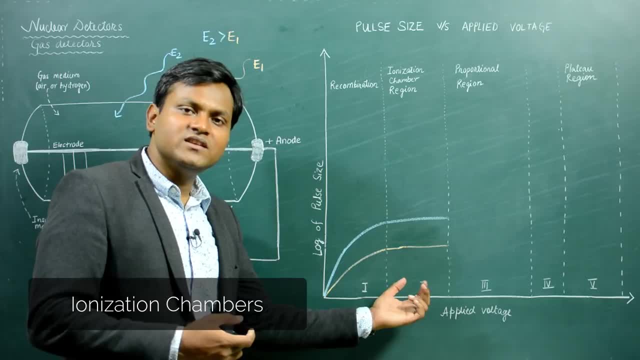 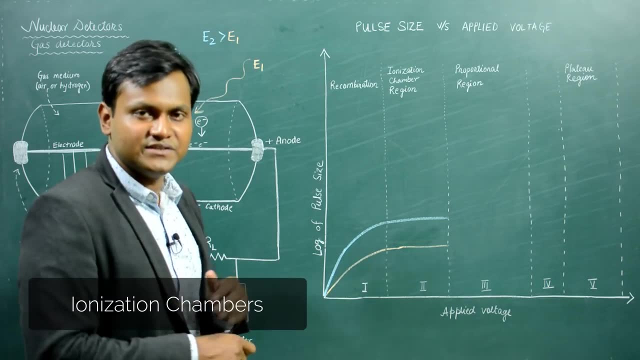 about zero, and any change in voltage within this region does not change the current pulse at all. rather, the size of the current pulse is purely dependent upon the kinetic energy of the incident particle. so greater the size of the current pulse, greater is going to be the kinetic energy of the 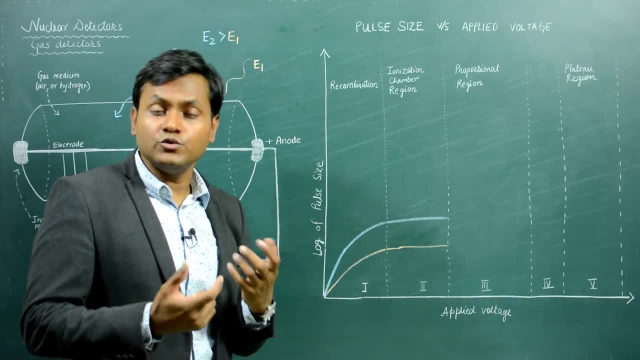 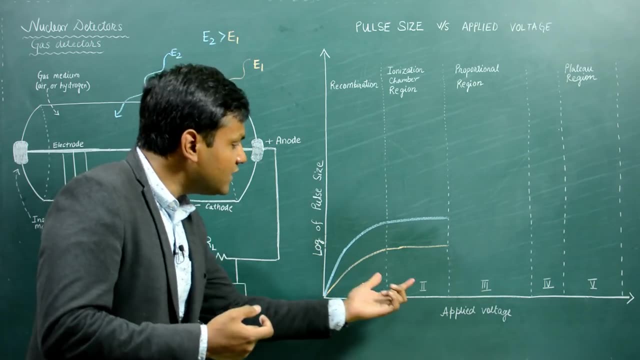 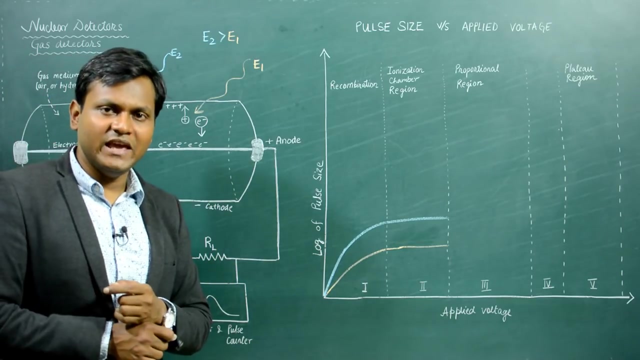 incident particle. this kind of a nuclear detector is basically used to detect high energetic alpha particles, beta particles or gamma radiation. now what is going to happen if we further increase the voltage of this particular system? if we further increase the voltage in this particular situation, a very different kinds of behavior, a different kinds of mechanism is seen. What happens? 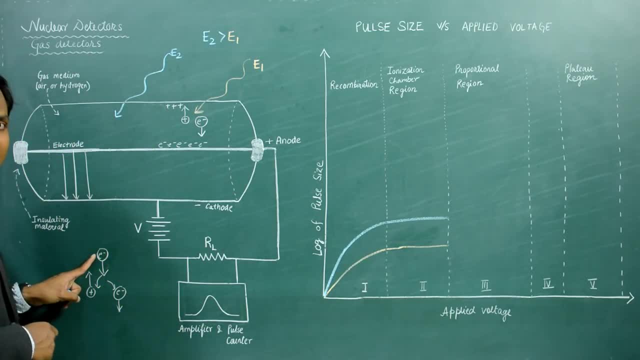 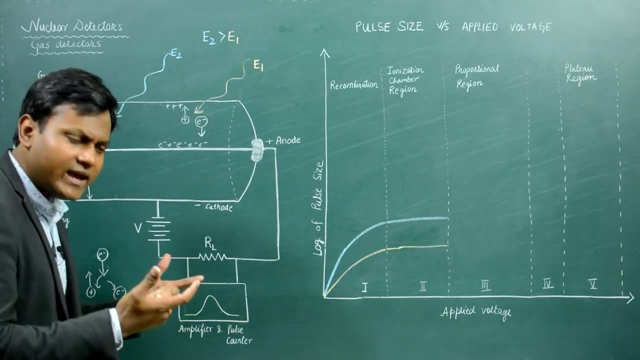 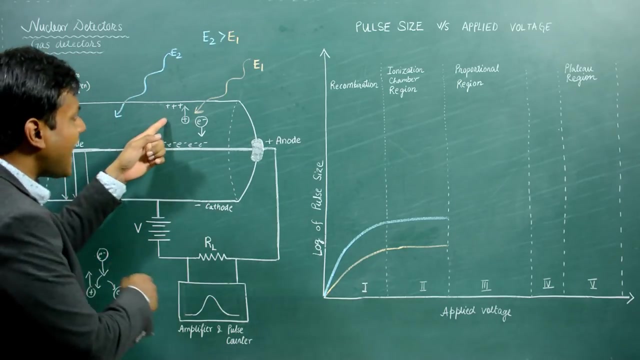 is that when electrons are created during primary ionization, they're accelerated towards a positive anode of the system. Now if the voltage potential difference is extremely high, then these electrons will also further lead to secondary ionizations. That means these electrons and ions when they get. 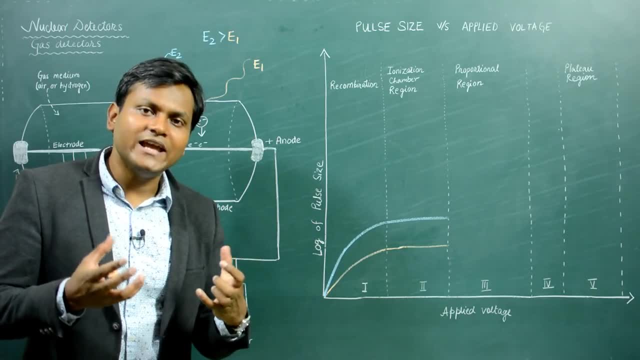 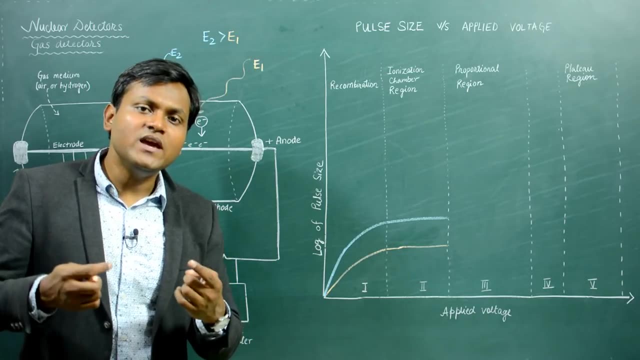 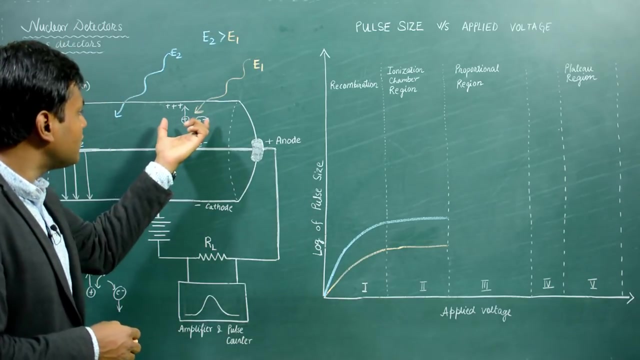 accelerated towards opposite polarities. they will also collide with the molecules of the medium and lead to further ionizations, which are known as secondary ionizations. So there is going to be a cumulative addition to the total number of positive ions and electrons due to secondary ionizations happening because of these collisions due to electrons and positive ions in the first. 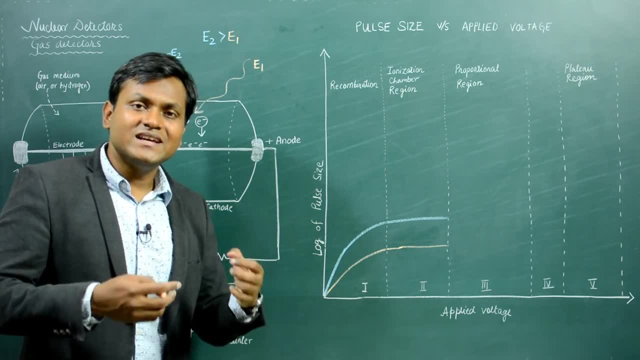 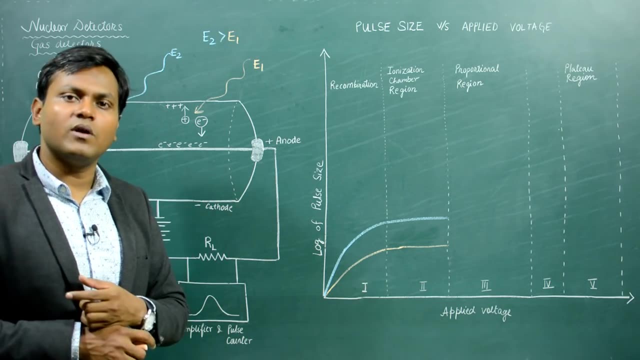 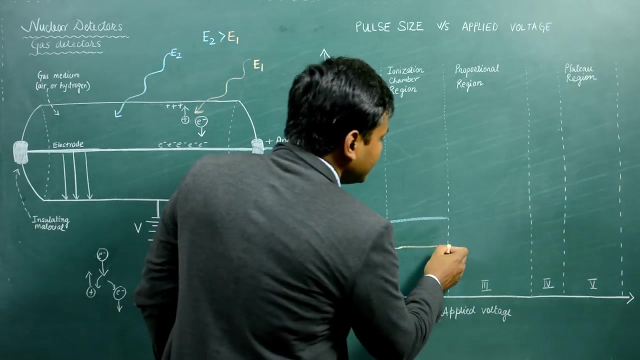 place. So as we increase the voltage further, the energy of the electrons and the ions become so high that they themselves cause secondary ionization, thus increasing the total number of ions and leading to an increase in the current pulse itself. What we end up with seeing is that the current pulse increases linearly with respect to voltage, So this is a 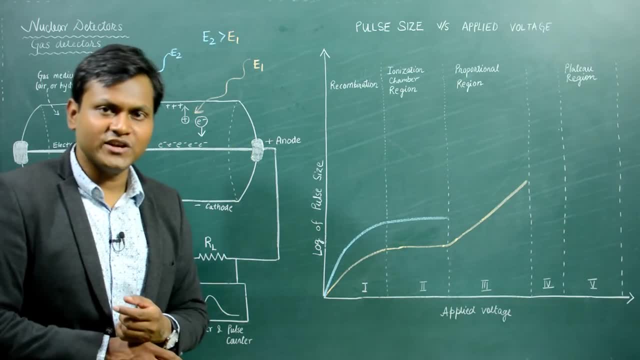 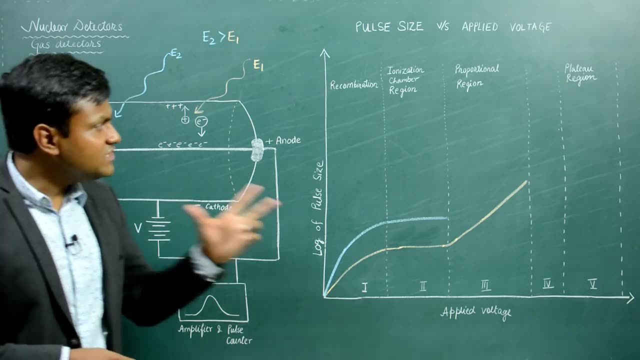 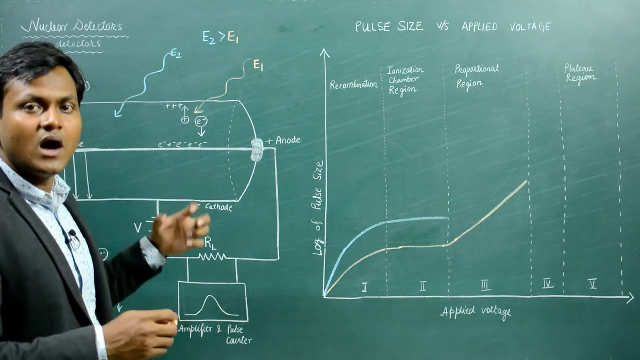 region of what is known as proportionality. So this is a proportional region where increasing the voltage leads to a proportional increase in the size of the current pulse itself. Now this region is very much important for low energetic nuclear particles, If the nuclear particles incident on this system are very less energetic and they are not able to induce sufficient amount. 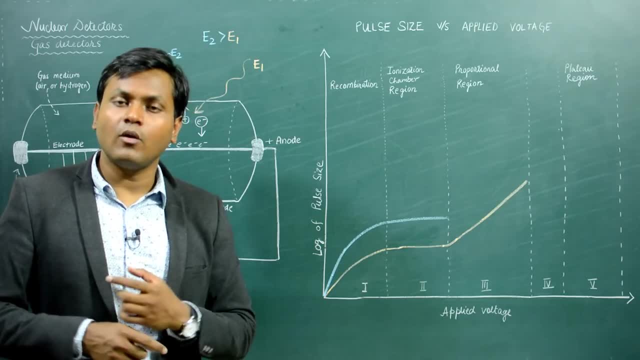 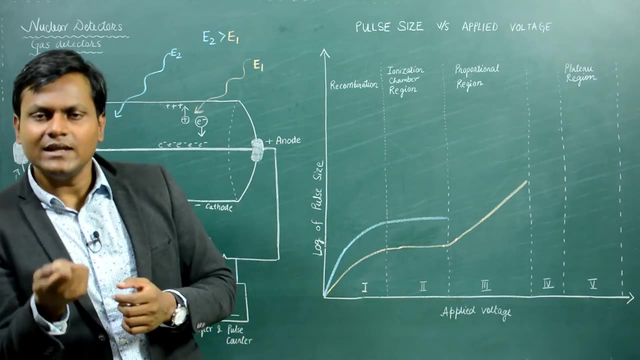 of ionization. then the current pulse itself will be so small that it would be difficult to differentiate from electronic noise. In those cases, for particles having very low energy, we want to increase the signal of the current pulse itself. In those cases it's better to increase the 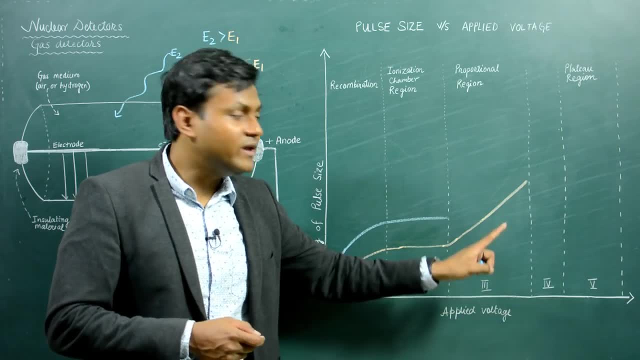 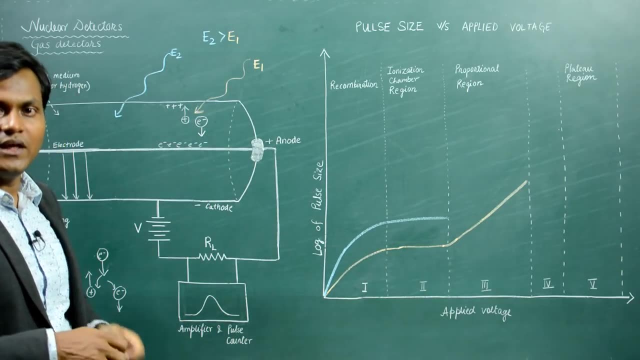 voltage, so that the current pulse itself will increase with the increase in the voltage and we can distinguish the current pulse from electronic noise. Now how can we distinguish two particles from each other for this particular region, Since there is a proportionality for both these two? 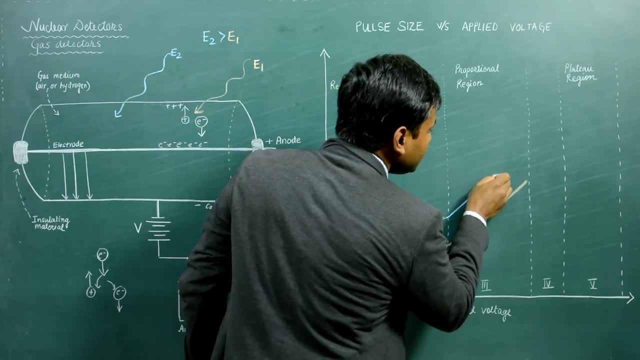 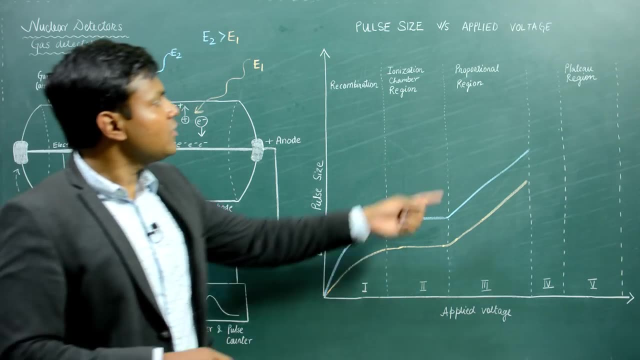 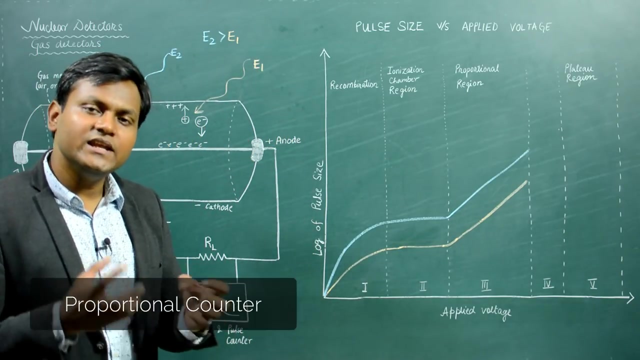 particles will have a current pulse which will increase proportional to the voltage, and we can distinguish between both of these two particles having different energies. So this is a region of proportionality, and the detectors which work in the proportionality region are known as proportional counters. They're basically used to detect less energetic particles where the 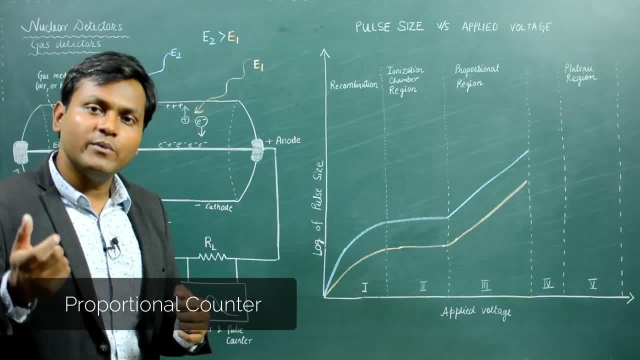 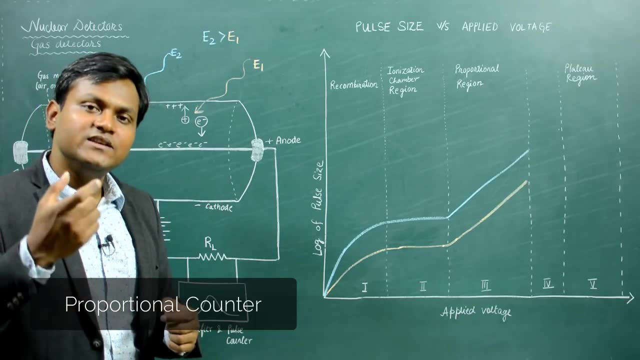 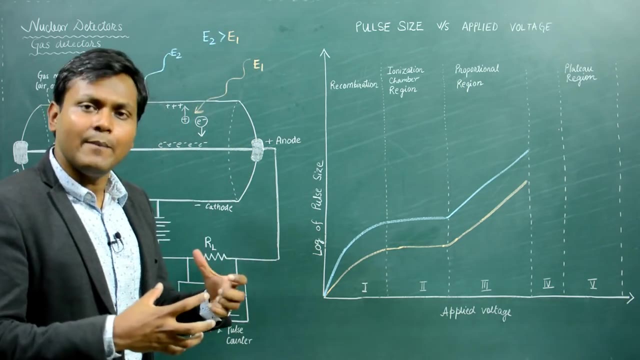 particles does not have sufficient kinetic energy to lead to primary ionization that can create current pulses which can be distinguished from electronic noise. We increase the voltage so that the primary ionization leads to secondary ionization and that leads to a cumulative increase in the size of the current pulse itself. What happens if we further increase the voltage? 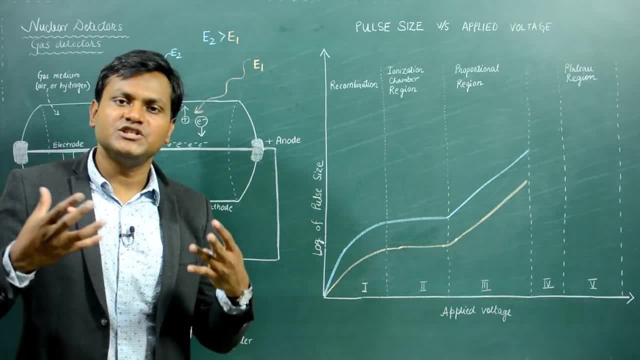 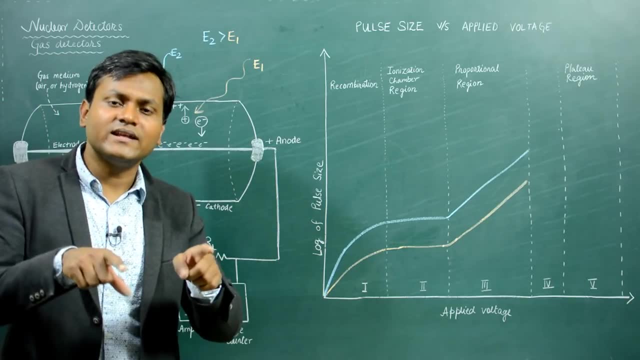 Further increase in the voltage will lead to a sort of an avalanche effect. The primary ion will create further secondary ions. The secondary ions will create further tertiary ions. They will create further ions. A chain reaction will happen which will lead to an avalanche effect. and this avalanche 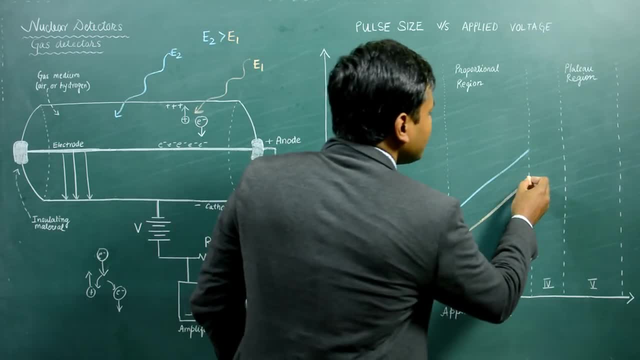 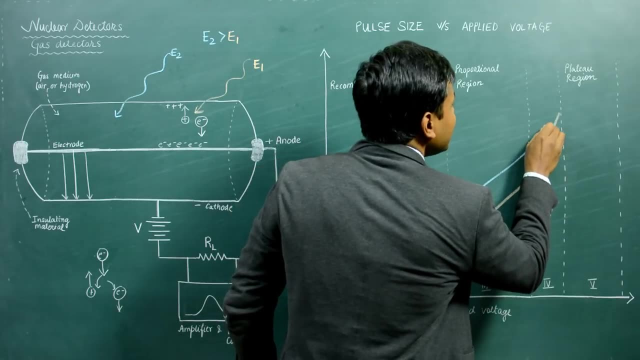 effect will increase the total number of ionizations happening. So what is going to happen is that we will have a region where there is a limited proportionality. That means the proportionality of the increase of the current pulse with respect to the voltage will be destroyed and we end up. 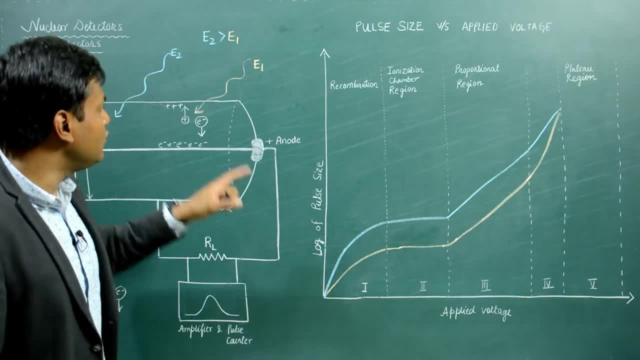 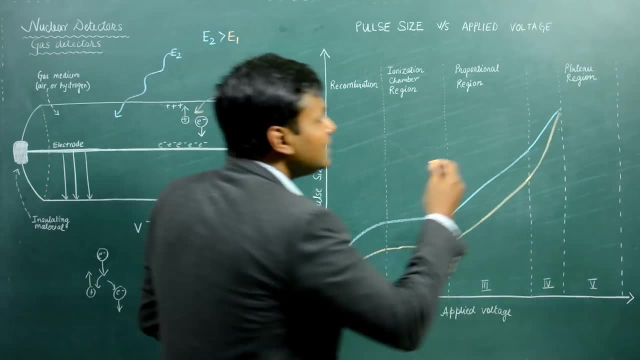 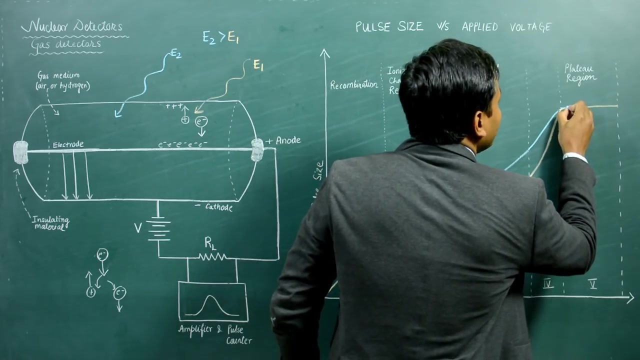 reaching a particular situation where, with sufficient voltage, even one less energetic electron can lead to an avalanche across the entire chamber of the nuclear detector, so that you end up getting what is known as the plateau region. So in the plateau region, even a small, less energetic particle can. 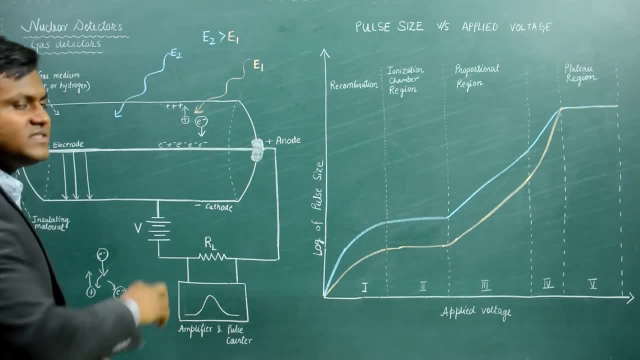 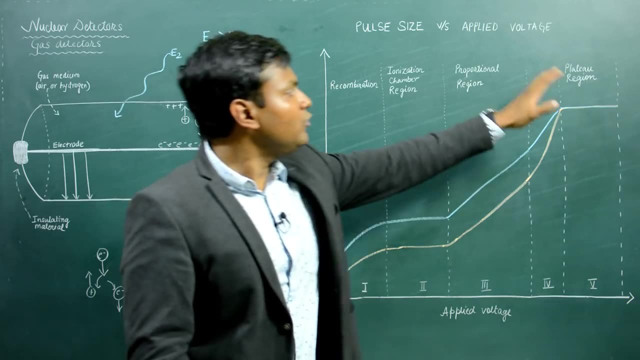 create an avalanche effect along the entire chamber itself, thus leading to a huge amount of current pulse corresponding to that particle. Now, as you can see, here in the plateau region we end up getting only one particular signal corresponding to ionization of the entire chamber. 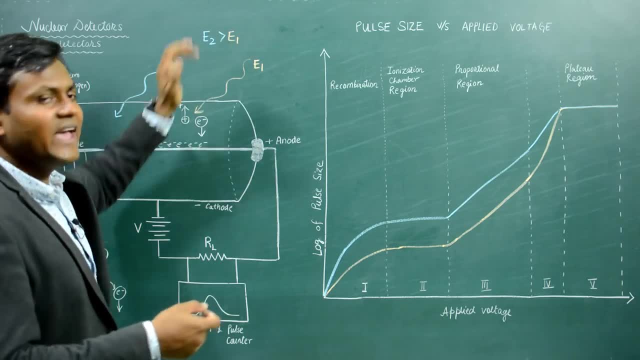 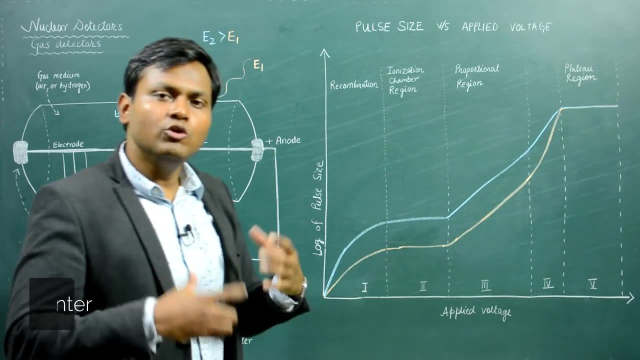 So therefore we cannot distinguish between a low energetic and a high energetic particle, because both of them will create the same amount of current pulse. So this region is basically known as the plateau region, and the nuclear detector which works in this region are called the Giegel-Müller counters. So Giegel-Müller counters cannot distinguish between the energy. 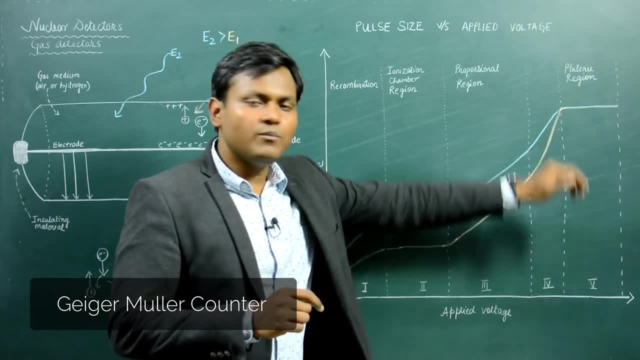 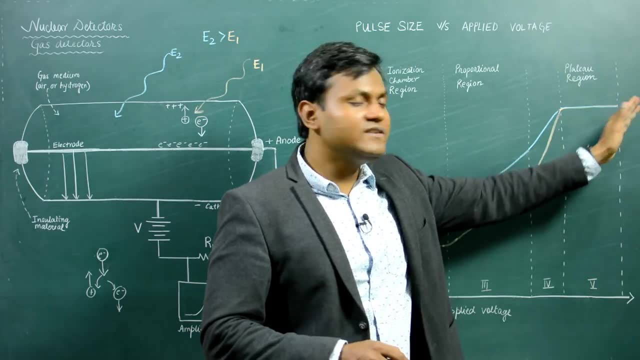 of different particles, but they are very good at counting the number of particles which enter a particular nuclear detector. Beyond this region we do not want to go, because further increase in voltage would basically lead to a situation where even the absence of any kind of a nuclear 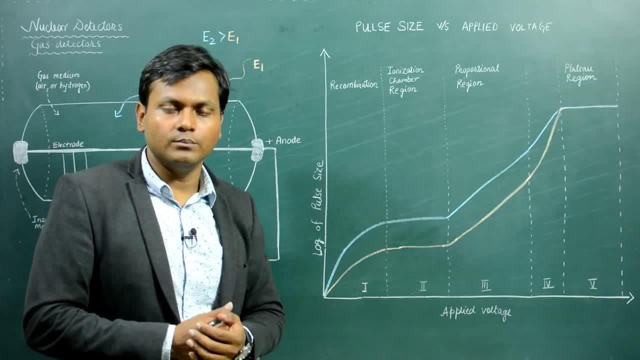 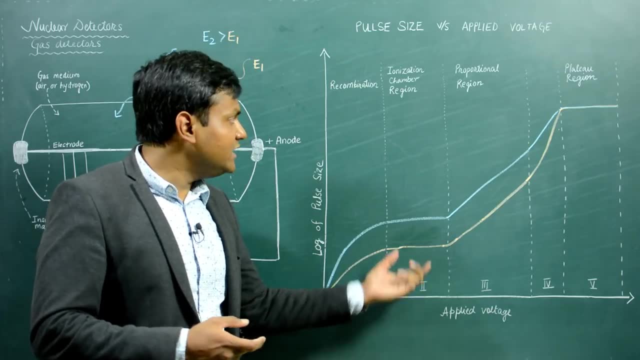 particle will lead to electric discharge, which is not favorable at all. So, as you can see from this graph, ionization chambers basically work in a region where recombination is very, very less and the ionization that is happening is a primary ionization. They are very good for detecting. 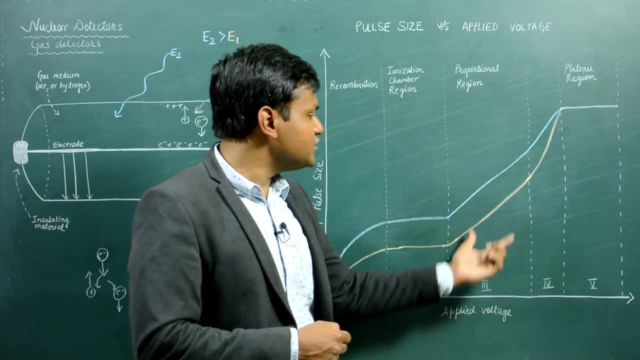 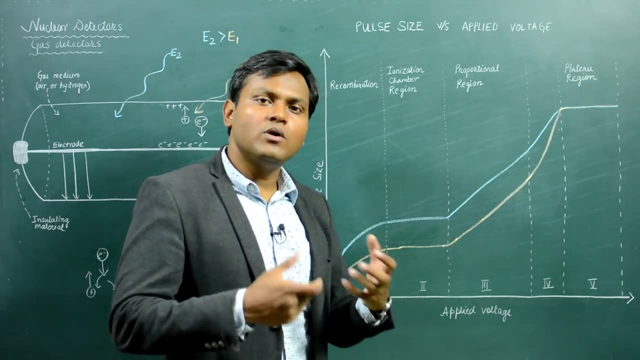 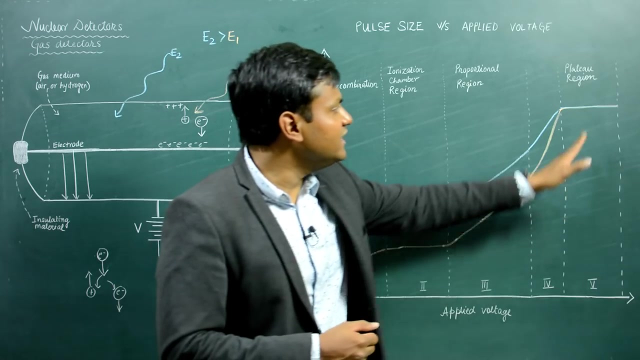 high energetic particles and proportional counters basically work in a region where there is a secondary ionization happening, but the secondary ionization is such that the increase in voltage would only lead to a proportional increase in the current pulse itself. This is basically a region used for detecting less energetic particles. and lastly, we have the Giegel-Müller counter region. 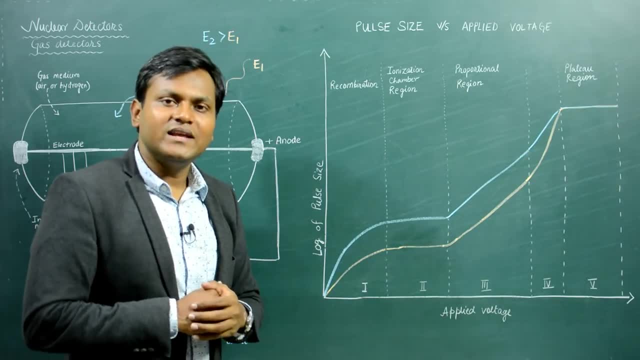 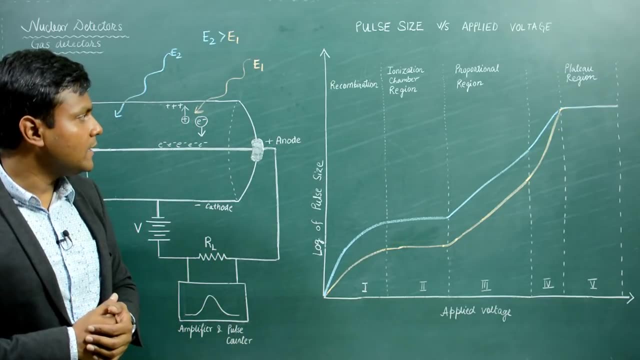 in which the presence of even a tiny particle having less energy can create an avalanche effect over. So that is all for today's discussion. I hope you have learned to distinguish between different kinds of nuclear detectors based on this graph. That's it for today. Thank you very much.